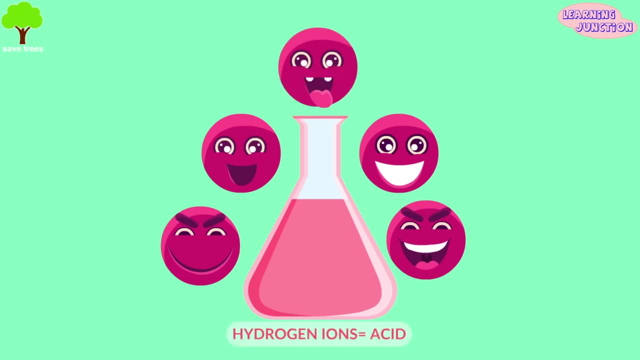 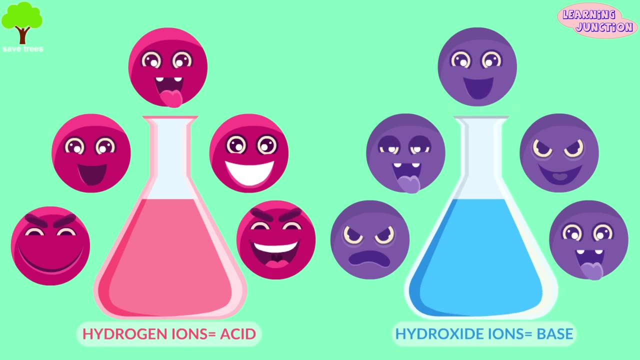 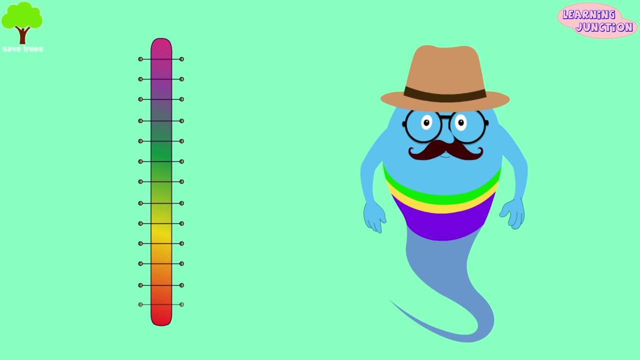 If it has so many hydrogen ions, then it's an acid. If it has so many hydroxide ions, then it's a base. It's that simple. See this scale. Scientists use this scale, called a pH scale, to check how acidic or basic a liquid is. The pH scale is a chemical detector. 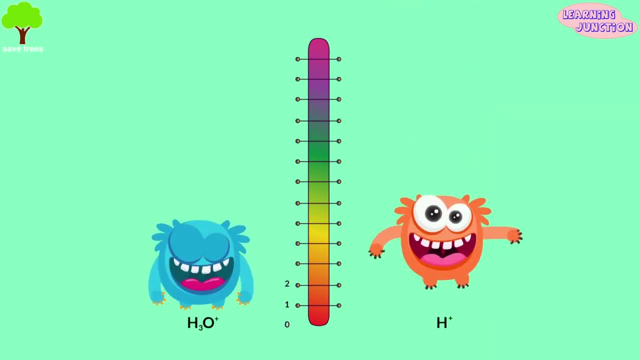 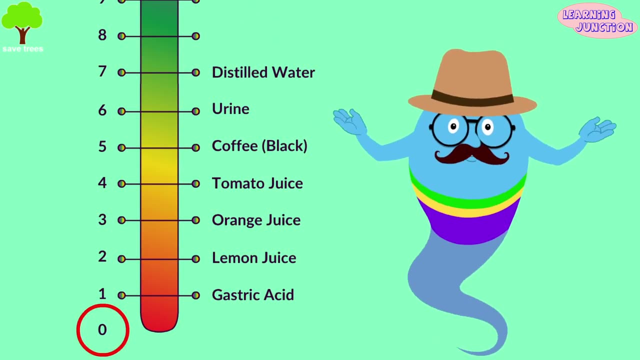 for hydronium and hydrogen ions, pH is a number ranging from 0 to 14.. What falls from a pH scale is a number ranging from 0 to 14.. From 0 to 7 are acids, with 0 being the strongest. Whatever comes within 7 to 14 are bases. 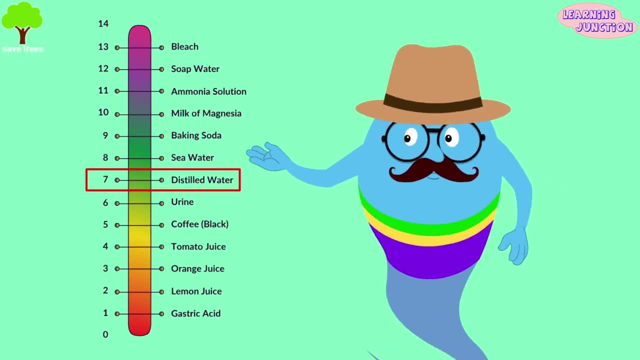 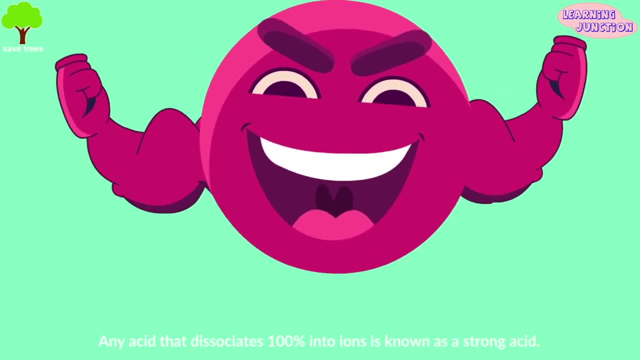 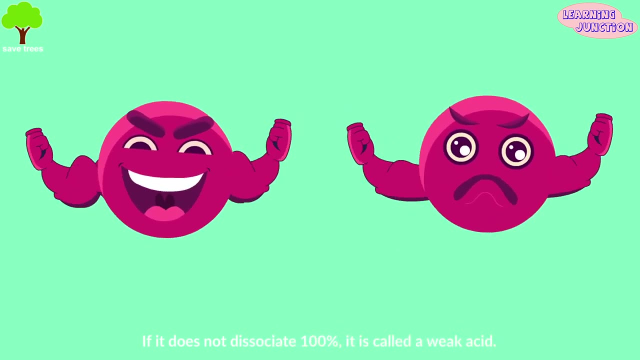 with 14 being the most powerful base. A liquid is neutral if it has a pH value of 7.. Any acid that dissociates 100% into ions is known as a strong acid. If it does not dissociate 100%, it's called a weak acid. There are a lot of 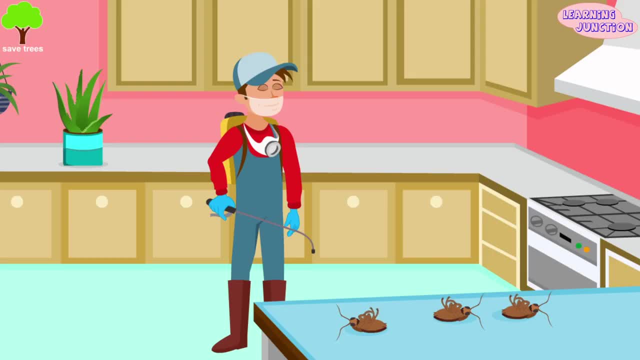 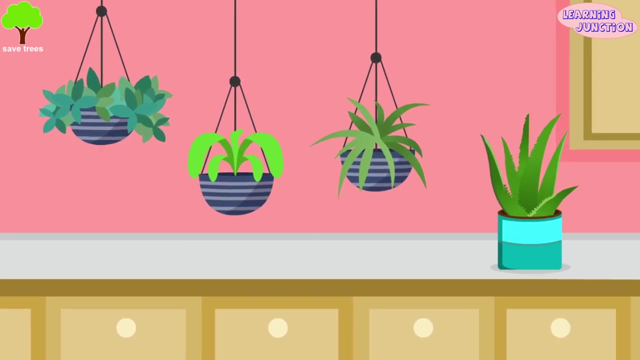 strong acids and bases in nature. Few of them, like boric acid, is used in insecticides. Some acids, like hydrochloric acid, is very dangerous, But some of them are so helpful. Many plants have acids and bases in their seeds and leaves. 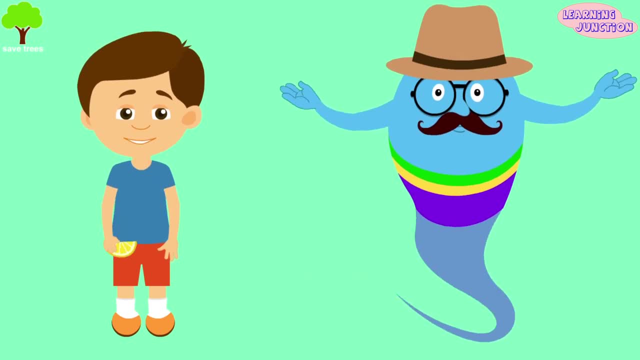 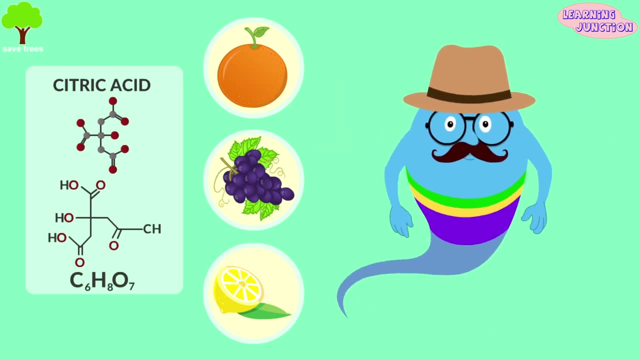 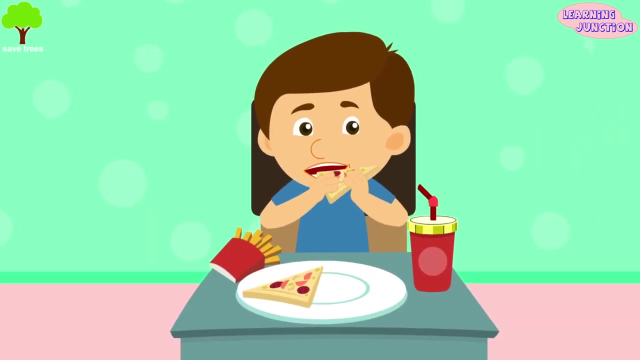 This lemon is so sour, my friend. Citrus fruits like oranges, grapes and lemons have citric acid in their juice. This is why lemons taste so sour. Let's see some uses of acids and bases. Remember when your stomach was upset after? 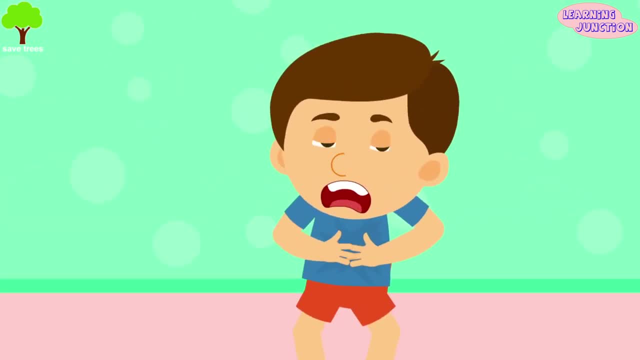 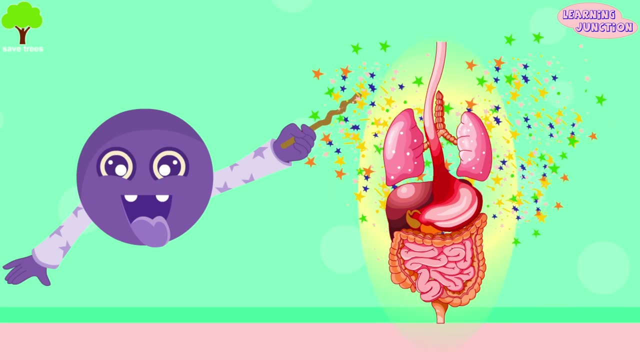 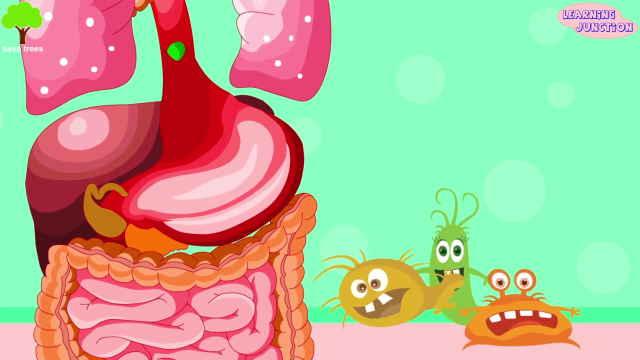 eating junk food. doctors gave you antacids. These include sodium bicarbonate or baking soda and calcium carbonate. They are bases and work by neutralizing stomach acids to water and carbon dioxide gas. The stomach uses hydrochloric acid to help in digestion. 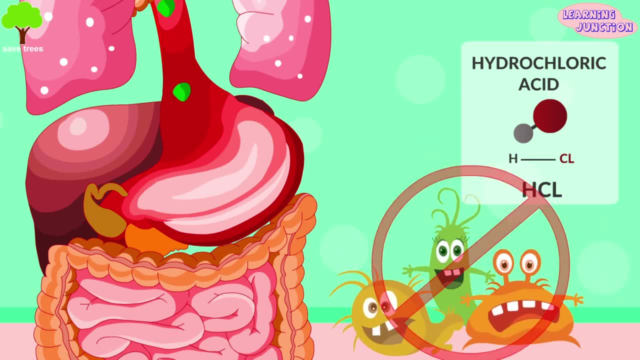 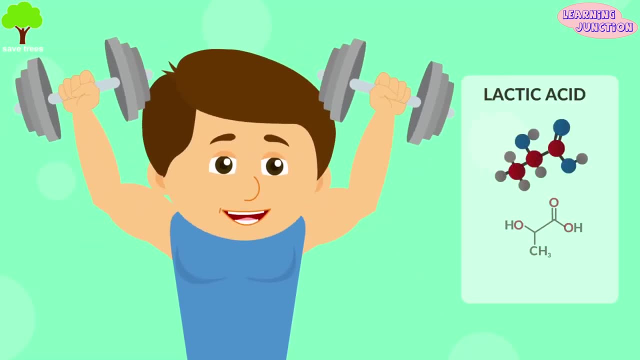 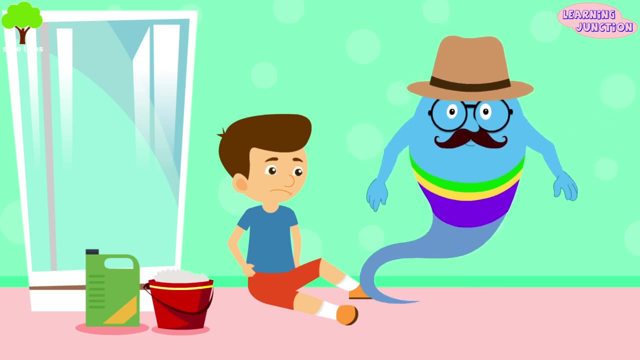 This strong acid also kills bacteria and keeps you healthy. Very good, buddy. When you exercise, muscles produce lactic acid. Oh, careful, There is cleaner in the floor. It is slippery. Bases feel slippery because these are soapy in nature.